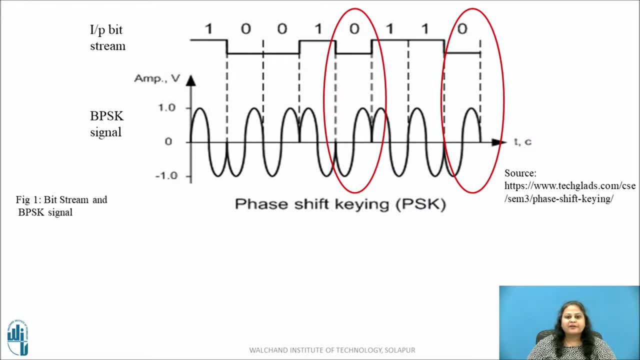 0 are represented with two phase angles separated by 180 degrees. The mathematical expression for PSK signal is expressed as shown. If carrier signal is given by A cos- omega Ct, then VPSK of t is equal to A cos omega Ct plus theta. Then. 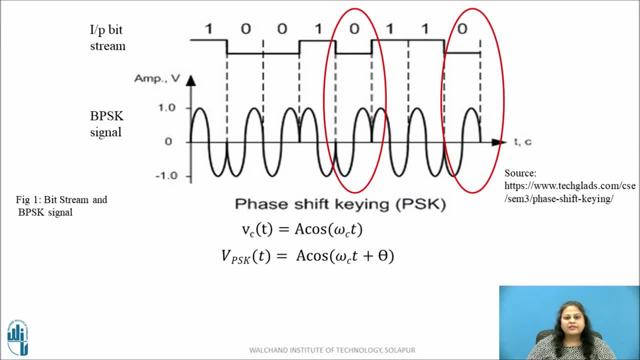 theta is 0 degrees and 180 degrees for input bit 1 and 0 respectively. Thus VPSK of t is equal to A cos omega Ct when input bit is 1 and minus A cos omega Ct when input bit is 0.. Also, from the waveform you can observe that BPSK is similar to amplitude modulation. 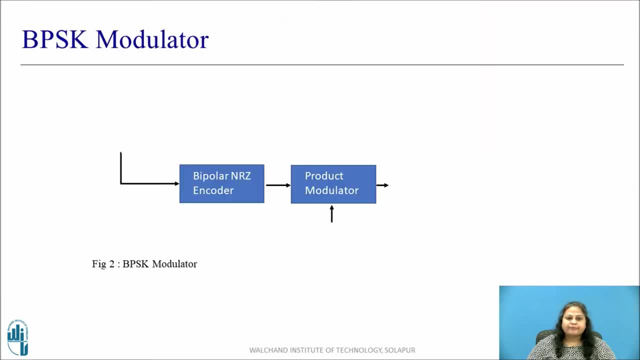 with modulating signal being digital signal. Let us now see how BPSK signal is generated. Figure shows the BPSK modulator. It consists of bipolar NRZ encoder and product modulator. The binary input sequence is first applied to the bipolar NRZ encoder. This output bipolar signal is then applied to one of the two inputs. 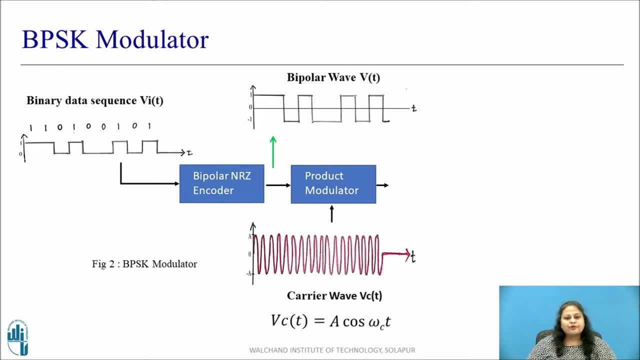 of the product modulator. When input of the product modulator a high frequency sinusoidal carrier signal is applied, which is given by Vc of t is equal to A, cos, omega, Ct. The output of the product modulator is BPSK signal as shown. Let us see its working in detail. When input bit is 1, the output: 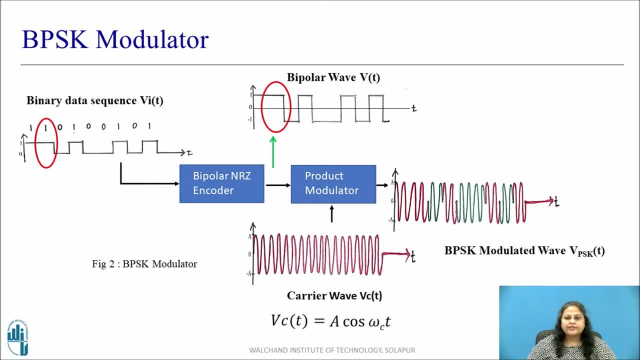 of the bipolar NRZ is a positive constant voltage, say plus 1 volt, which is multiplied with the carrier A cos omega Ct during the bit slot in product modulator. Thus the output during that bit slot is given by Vpsk of t is equal to A cos omega Ct. Thus the carrier 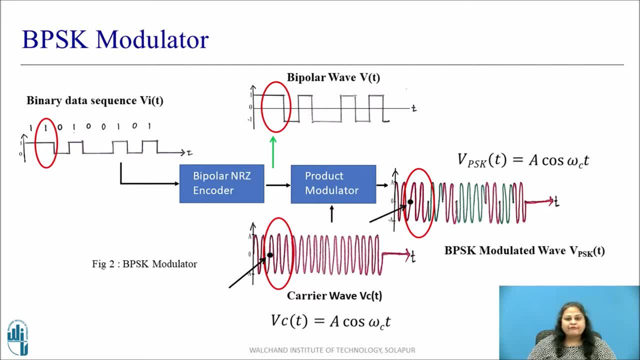 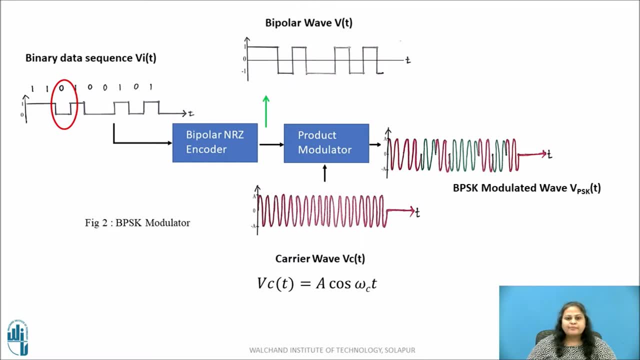 signal and the BPSK signal. they are in phase with each other, giving 0 degrees phase shift When the input bit is 0, the output of bipolar NRZ encoder is given by BPSK of t is equal to A, cos, omega, Ct. . . . . . . . . . . . . . . . . . . . . . . . . . . . . . . . . . . . . . . . . . . . . . . . . . . . . . 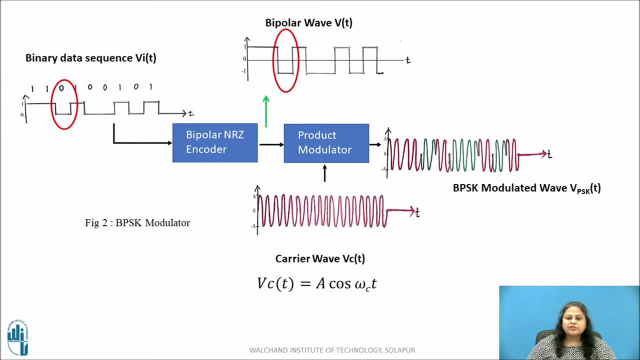 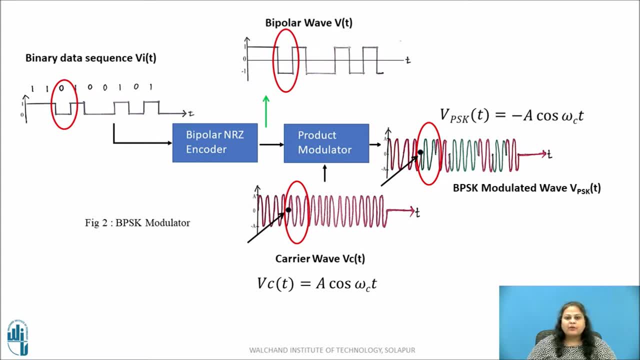 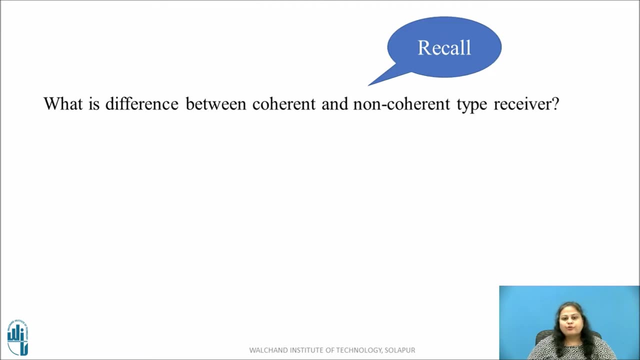 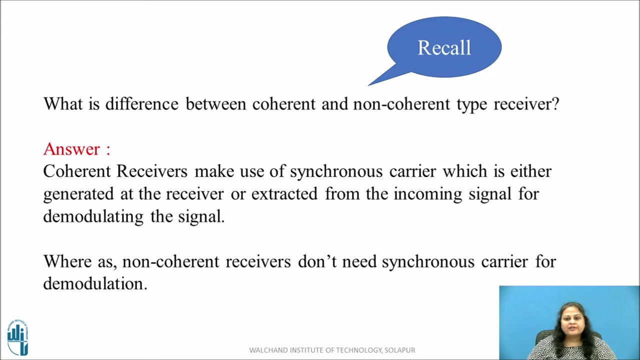 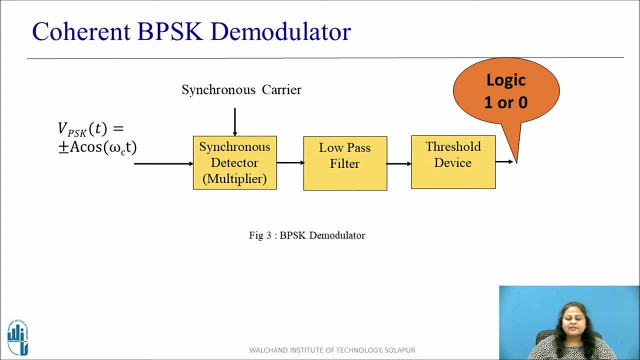 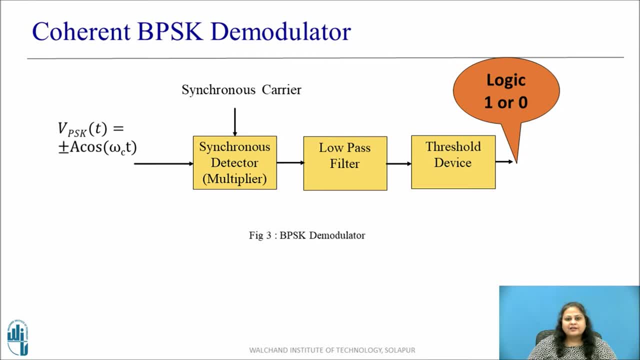 consists of a synchronous detector, that is, a multiplier, low pass filter and threshold device. The incoming BPSK signal is equal to plus or minus A cos. omega CT is applied to one of the input of synchronous detector. To another input, synchronous local carrier is applied which is either generated at the receiver or extracted from the incoming BPSK. 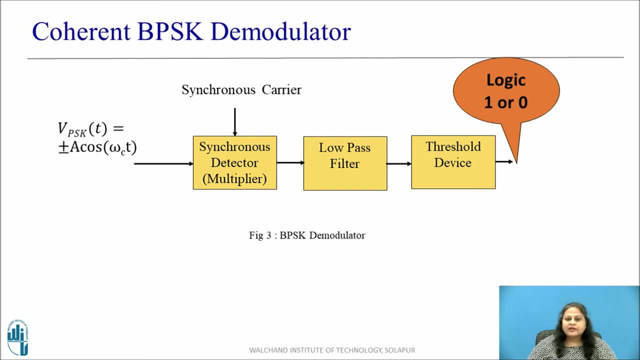 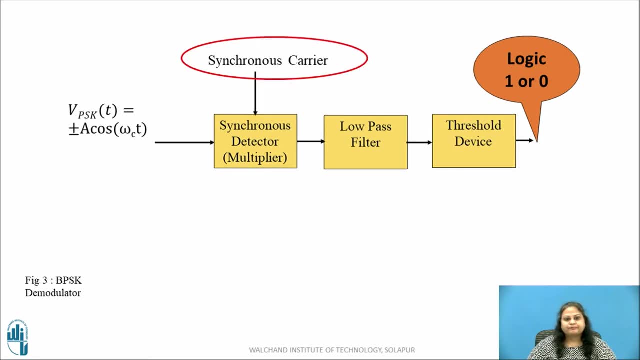 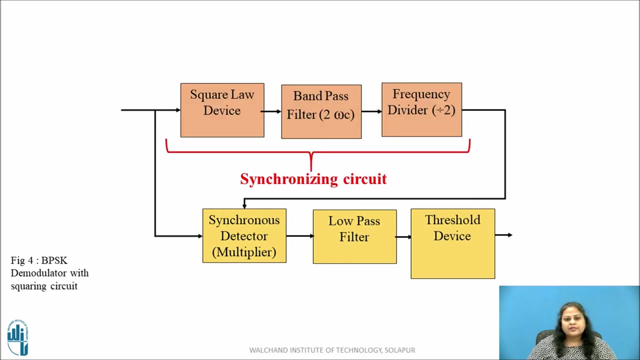 signal. Finally, the demodulated information bit stream is obtained at the output of the threshold device. Also, the synchronous carrier signal in coherent BPSK is extracted from the received signal. For this a synchronizing circuit is used as shown. The synchronizing 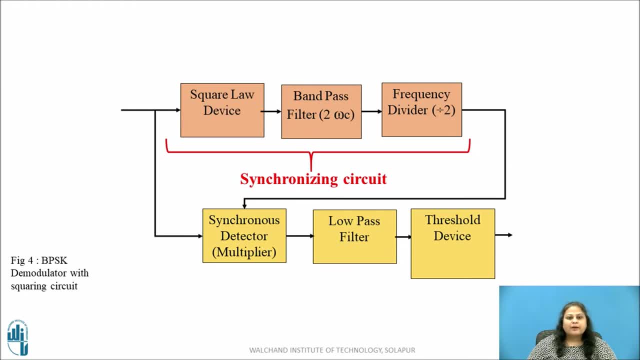 circuit consists of a square law device, band pass filter and a BPSK. The received BPSK signal is applied to the square law device and the output of a frequency divider is the extracted synchronous carrier. Let us see its working in detail During a 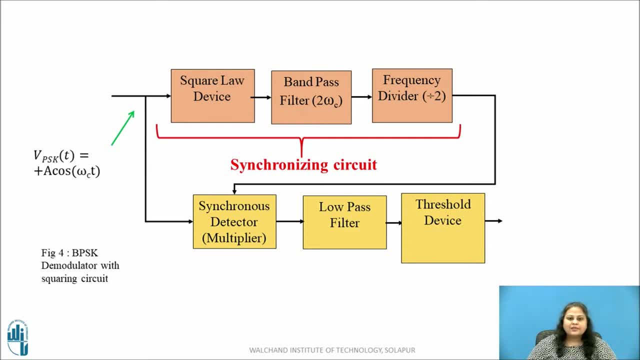 bit slot when the incoming BPSK signal is plus A cos omega CT. the output of square law device, which is also known as squaring circuit, is A square omega CT divided by BPSK. The signal is then passed through a band pass filter which is tuned to twice omega C angular. 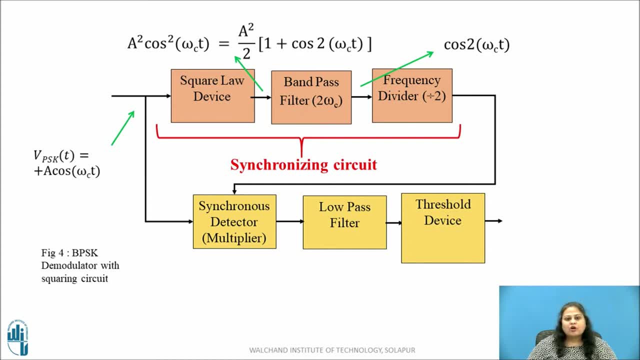 frequency. Thus output is cos2- omega CT which after division gives the required synchronous carrier cos of omega CT. Now in the synchronous detector, the signal is passed through a band pass filter which is tuned to twice omega C angular frequency. Thus output is cos2- omega CT which after division, 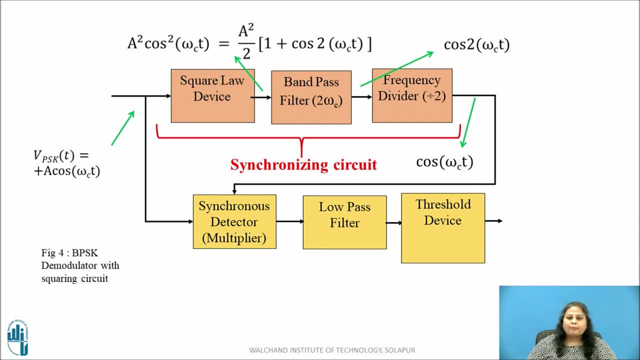 gives square law. VW1m 2 Sonic bpskesta. The locally recovered synchronous carrier, is multiplied with the received BPSK signal. The output of a synchronous detector is ACOS squared omega CT, which is then passed to the low-pass filter. The output of filter is thus a DC term plus A by 2.. This voltage is then: applied to a threshold device. This is then used togue on BPSK to take root and the output for Al-OZ field type counter вид angle looks like this: A cos2 omega CT is the output from the consistently recovered synchronous carrier which is: then passed to BPSK As a filter of frequency. it also identifies very suspected factors as load spread relation with BPSK. here A cos square omega Ct which was passed to BPSK here is then passed to BPSK, So slope of counterer, which is then yolks A cos square omega CT As way我們. 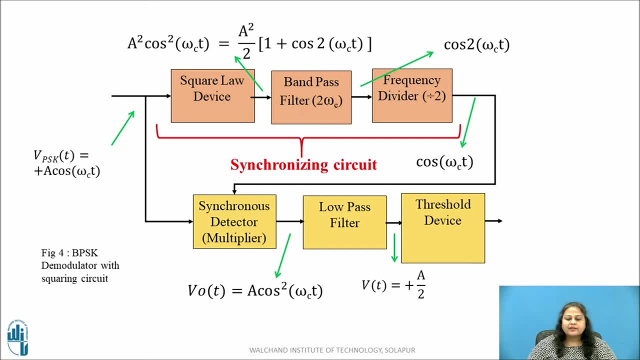 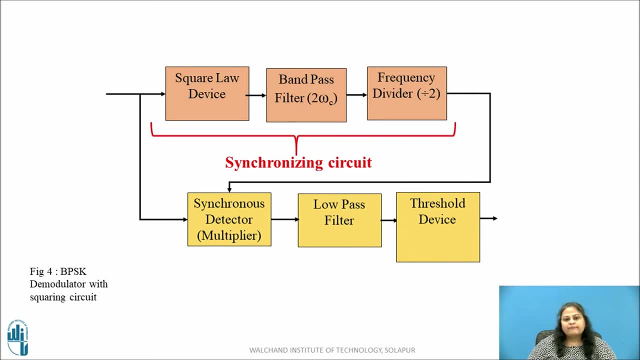 this voltage plus A by 2 is greater than the threshold value, the device gives an output logic 1.. Similarly, during the bit slot, when the received BPSK signal is minus A cos, omega CT, the extracted local synchronous carrier is again cos of. 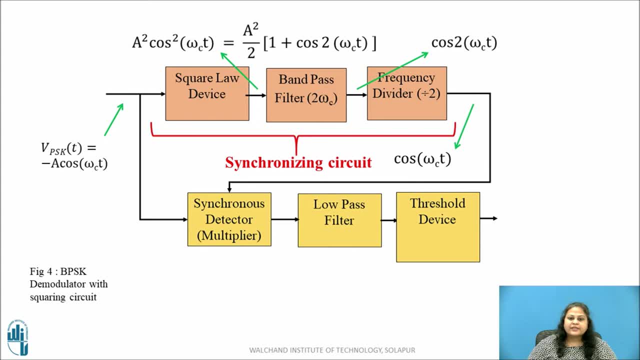 omega CT as shown. This received BPSK signal and the recovered local carrier is then multiplied in a synchronous detector. The output of synchronous detector is now minus A cos square omega CT which, on passing through the low pass filter, gives a DC term minus A by 2.. Now this voltage. 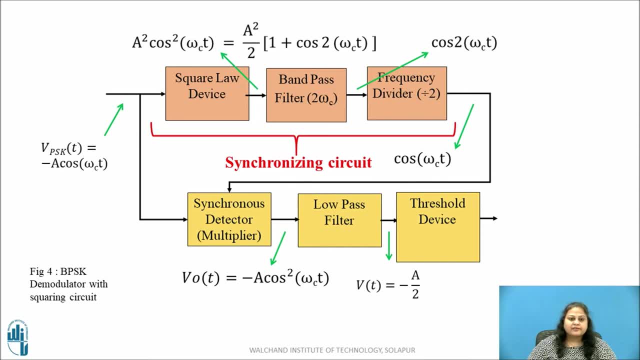 is less than the threshold voltage of the threshold device. Thus the output of threshold device is greater than A cos. omega CT is now logic 0. Thus it can be seen that during the bit slot, when input BPSK signal is A cos omega CT output is logic 1 and when input is minus A cos omega CT output is logic. 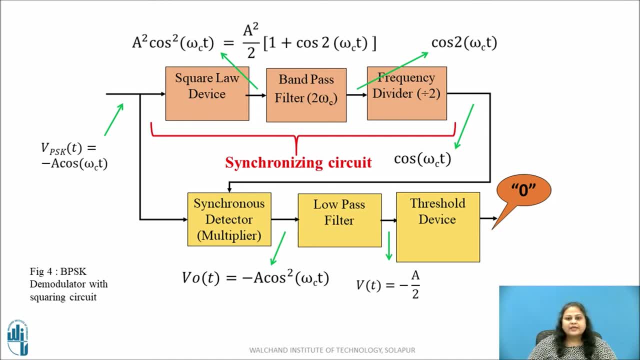 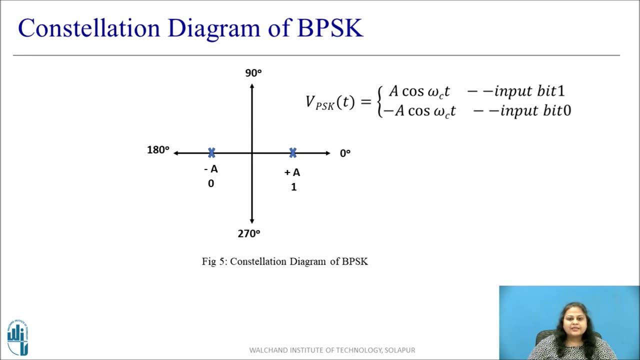 0.. This is how coherent BPSK demodulator works. Its major disadvantage is that it needs complex synchronizing circuit. Figure shows the constellation diagram of BPSK signal. It can be seen that BPSK signal is represented having two signals, with amplitude A and phase angle: 0 degree. 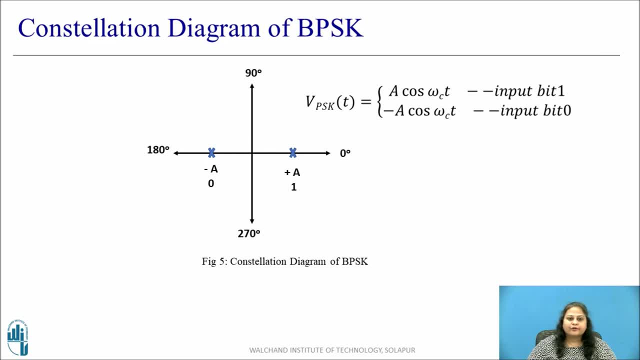 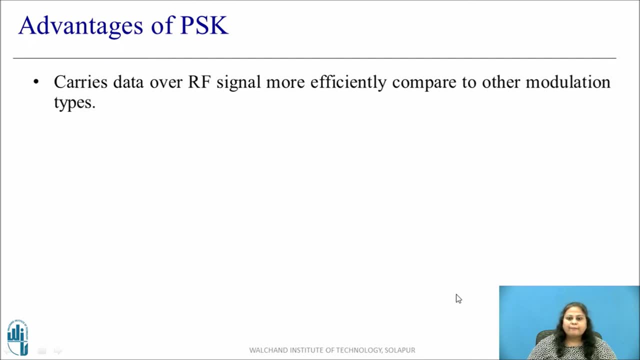 and 180 degree for bit 1 and 0 respectively. Let us see advantages of PSK signal Compared to other modulation techniques. PSK carries data over the radio frequency signal more efficiently, Even though it occupies same bandwidth as ASK. compared to ASK, it is less susceptible. 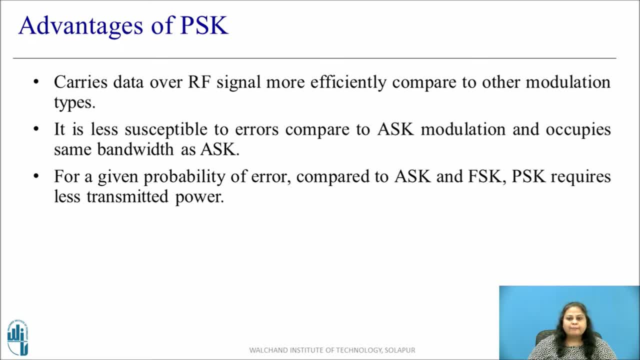 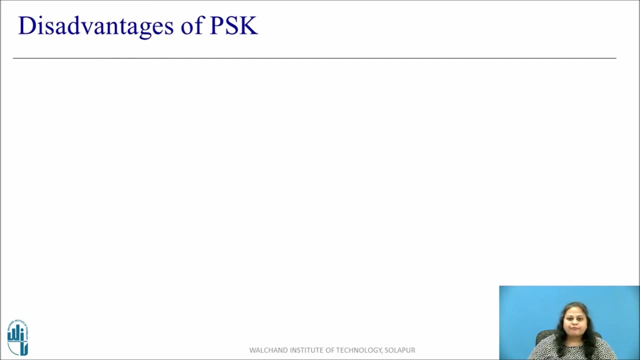 to noise. For a given probability of error, PSK requires less transmitted power. High data rate of transmission can be achieved by using higher level of PSK modulation. Let us now see disadvantages of PSK signal. PSK receiver is more complex than ASK and.